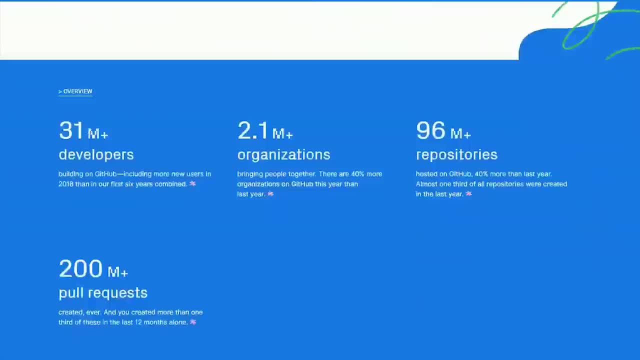 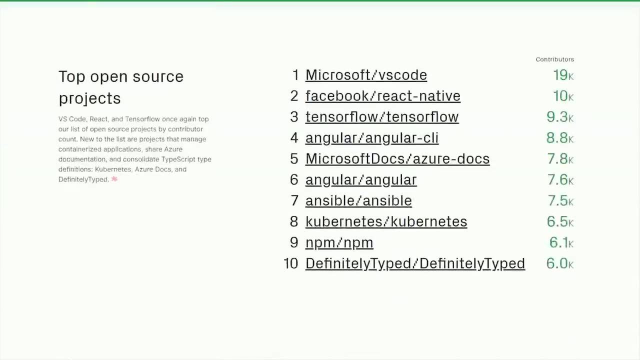 software world. It's essentially a history book of your code, and services like GitHub make open source software accessible to the world. In today's video, I'll show you the basics of Git, along with some advanced pro tips, and I'll even invite you to collaborate with me on a pull request on GitHub. 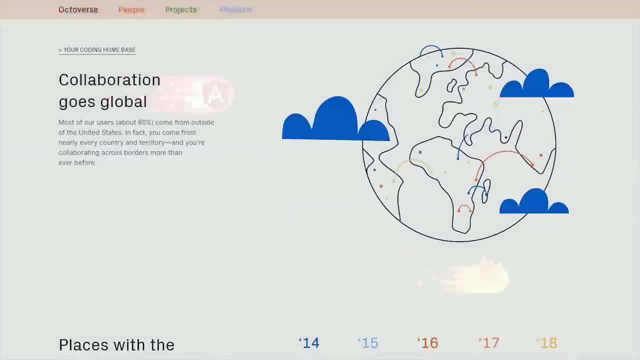 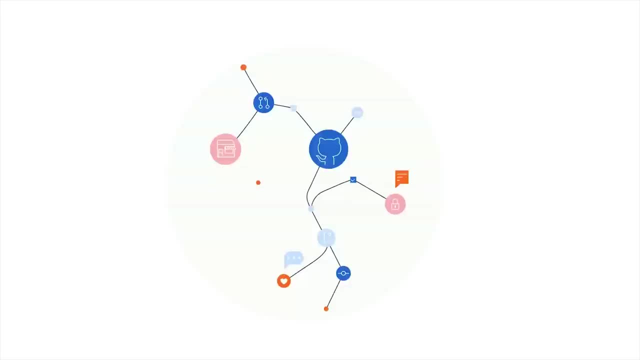 in exchange for a free sticker. I think that's a pretty good deal, so if you're new here, like and subscribe and I'll give you further instructions throughout this video. So what is Git exactly? It's a version control system, but really what that boils down to is a system for managing. 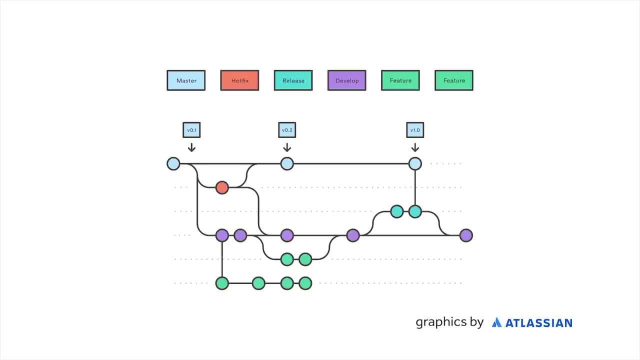 your files. Building software is a series of small milestones, where each milestone is just writing code in a bunch of different files. Your app will constantly move from a state of chaos to stability, and Git gives you a way to keep track of all of these changes, And it does so in a way that allows 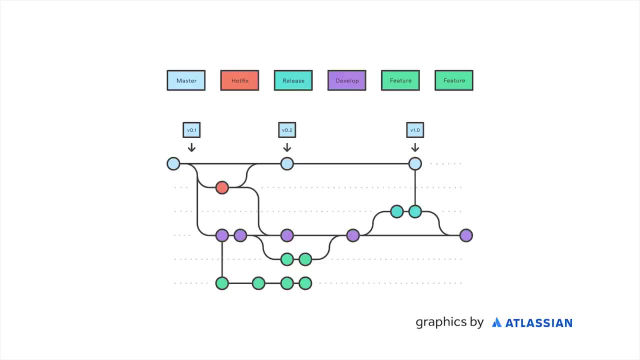 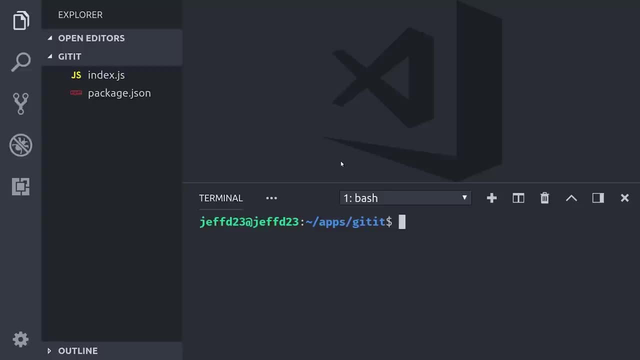 you to create multiple branches or paths that you can go down and then merge them in later, facilitating collaboration between large groups of developers. So today I'm going to show you how this all works by building a piece of open source node software that we can all collaborate on. 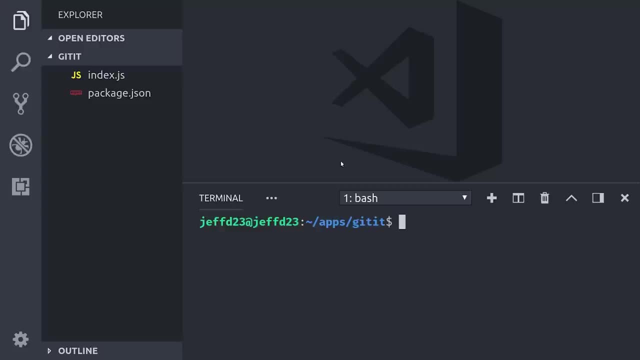 The software itself is a command line utility that will allow you to encrypt your mailing address and then add it to the GitHub repo so I can mail you a sticker. In my current working directory I have a command line utility called git init, and I'll go ahead and run git init from the command. 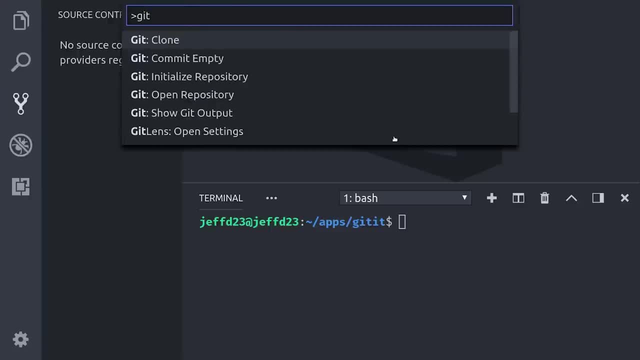 line and you'll see that it initializes an empty Git repository. So I'll go ahead and click on the source control icon and you'll notice it says no source control providers registered. The first thing we'll need to do is initialize Git to start tracking our files, and there are two ways we can. 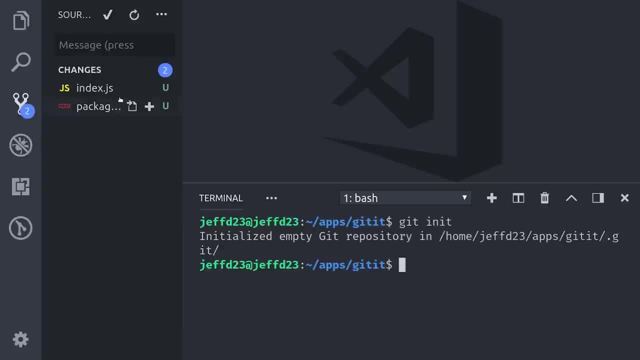 do this? We can either do it directly in VS code or we can do it from the command line. You should definitely try to memorize all the commands I show you in this video, but it's often faster to run them with VS code's integrated tooling, and I'll show you both methods throughout this video. 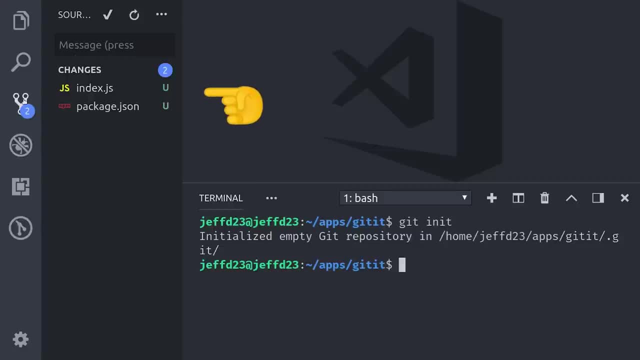 So let's go ahead and run git init and I'll show you how to do it in VS code. So let's go ahead and run git init and I'll show you how to do it in VS code's integrated tooling. So let's go ahead and run git init and I'll show you how to do it in VS code's integrated tooling. 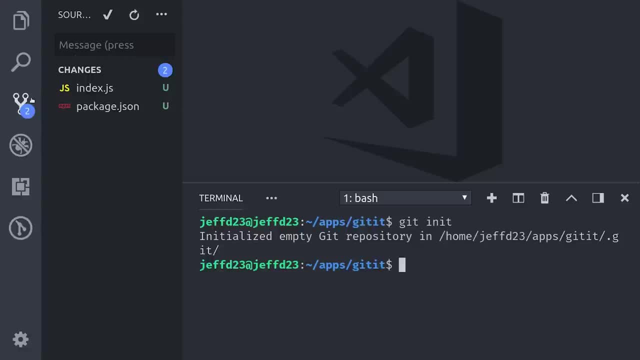 Because we're in a brand new project. both these files have a U icon, which means untracked or that they're newly created on this working directory. Now a quick pro tip: when you initialize a Git repo, it creates a hidden Git directory. If you want to completely uninitialize Git or remove it from your project, you can just remove. 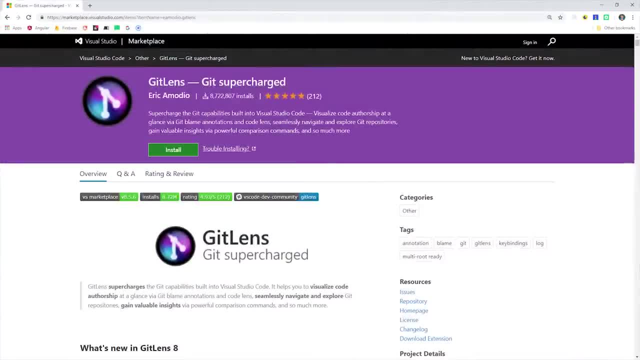 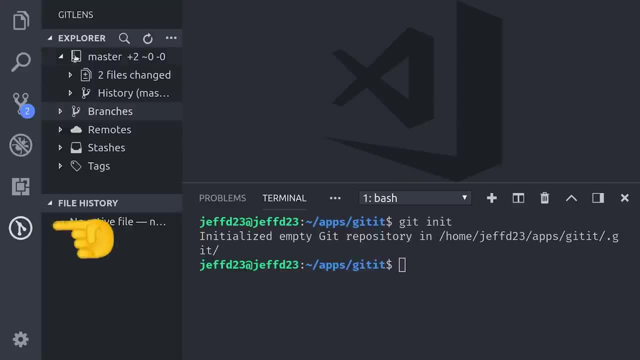 that directory, but be careful with that one. Now. a second pro tip is to install the Git lens plugin for VS code. It embeds all kinds of useful information directly in your code and gives you this extra panel where you can easily navigate your Git history. 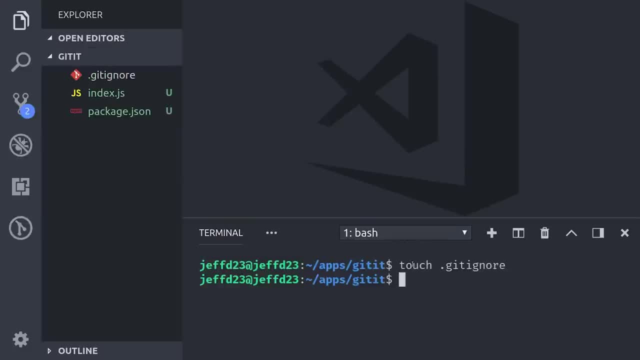 The next important thing when setting up a GitHub repo is to create a gitignore file. You don't want everything in source control. For example, you definitely want to keep out any sensitive private API keys, and you'll also want to filter out the source code for your dependencies, like your node modules and any unnecessary log. 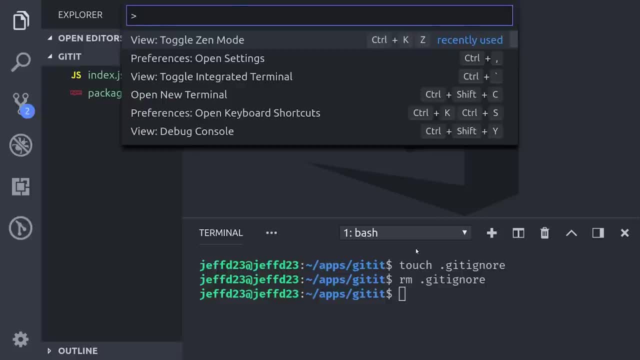 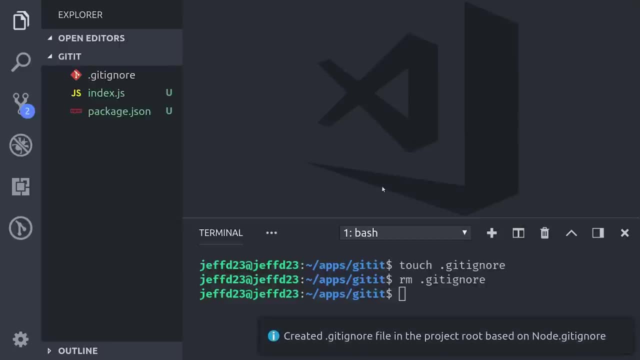 files. Git will automatically look at this gitignore file And filter out anything that matches the file path or pattern. You can create this file manually, but the pro way to do it is to use a VS code plugin to automatically generate all the defaults for your environment. 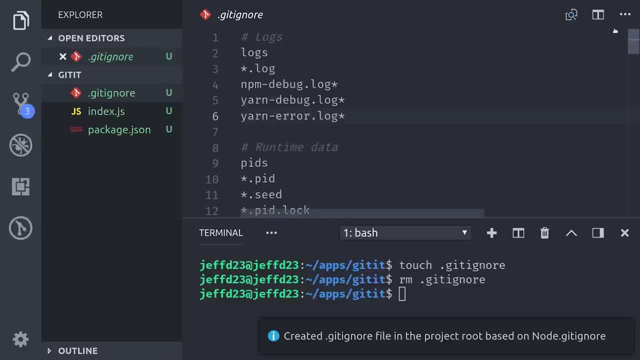 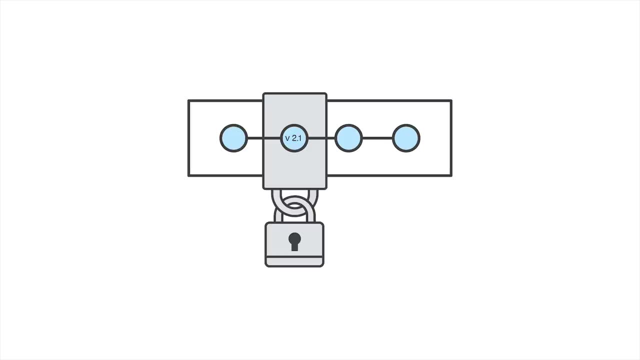 So that saves us a bunch of time. and now we can move on to the next concept of how do I take a snapshot- or commit- of my current working directory. A commit is like a page in the history book that has its own unique id and can't ever be changed without Git knowing about it. 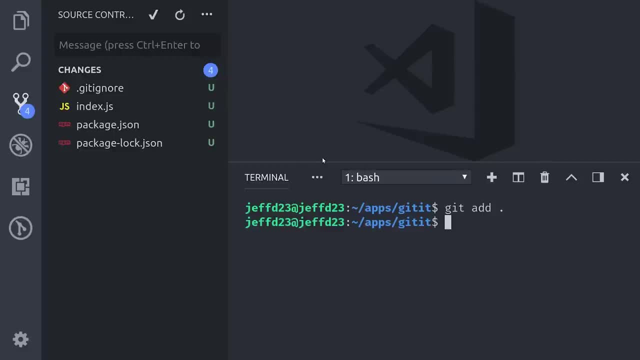 The first thing we'll want to do is stage the files that we want included in this commit. You stage files by running git add and you can add individual files or the entire working directory by just using a period, And VS code makes it really easy to stage or unstage files by just clicking the plus or minus. 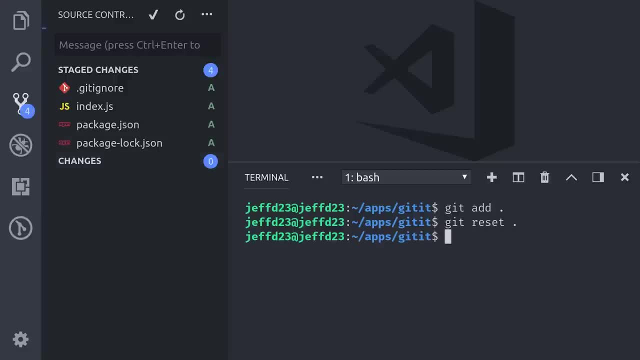 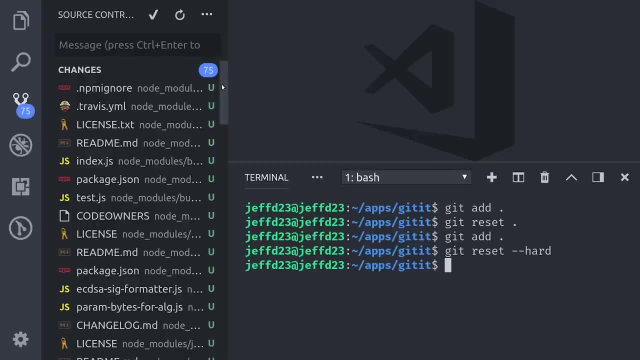 button And you can unstage files from the command line by running git reset. But be careful with this one, because there's a hard flag and if you use it it will not only unstage the files but delete them forever. So if we run that one right now on our new project, it will delete everything and we'll 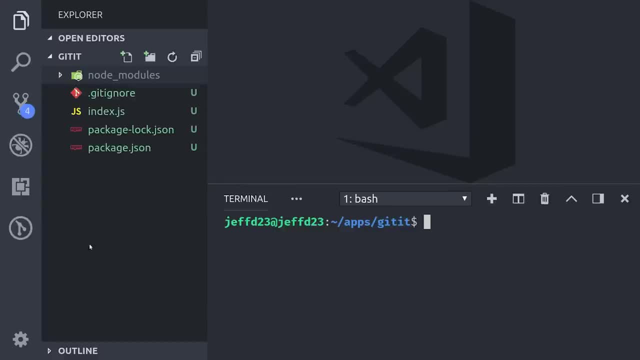 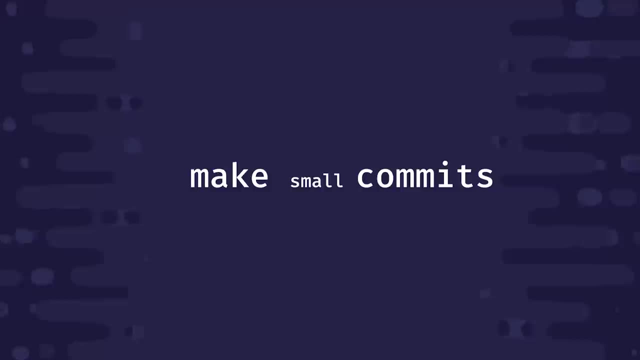 have to start over from scratch. And with that I'll give you one of my most useful tips, My most important pro tips, which is to make many small commits. This practice will not only help prevent catastrophic losses of code, but it will also just make your code changes a lot easier to follow. 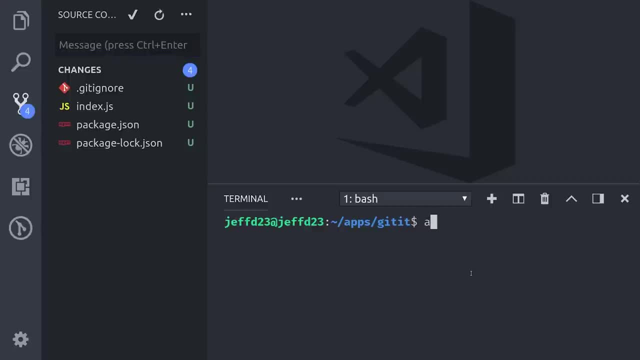 Now we're ready for our first commit. The first thing we'll want to do is run git add to stage our files. Then we run git commit with the m flag to add a descriptive message about what we changed in our code. A pro tip here is to use an emoji to get more github stars on your project. 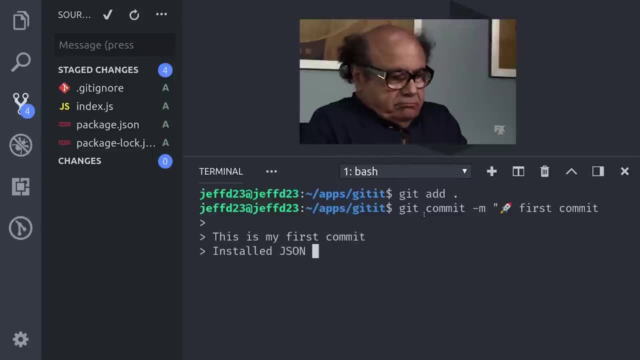 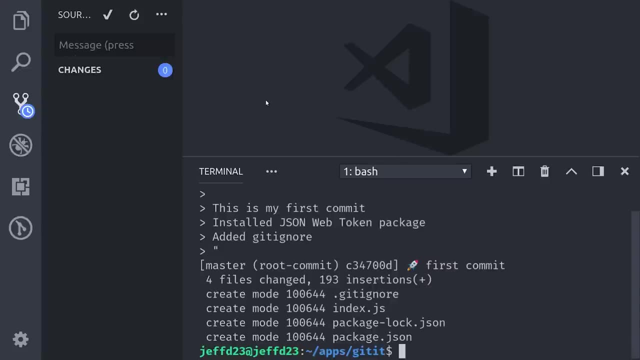 Because github stars are the best way to tell how good a software project really is, And you can also make your comments multi-line, to provide a summary on the first line and then a more descriptive set of changes on the second line. You'll notice that that takes the files out of the stage changes and gives us a clean. 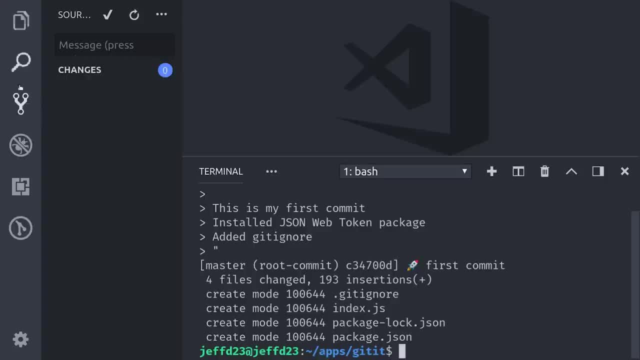 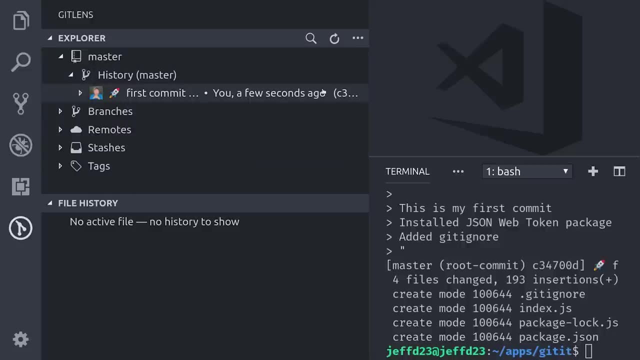 working directory And git will tell us exactly which files were created, modified or deleted as part of this commit. Now if we go into our git lens plugin, you can see we have a history of code changes that we can navigate through and see exactly which lines of code changed. 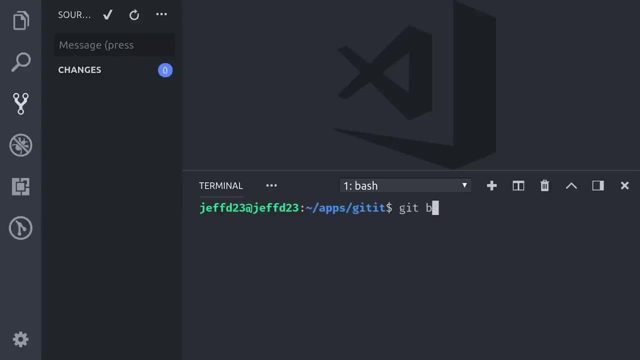 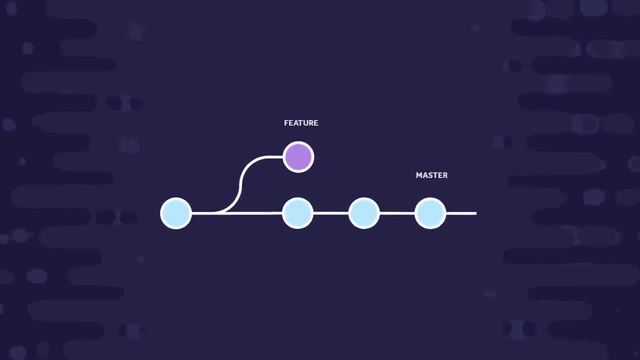 Up until this point, we've been working on what's called the master branch, Which is like the main trunk on the tree That contains the actual source code that you're releasing and delivering to your customers. So what happens when you have a stable codebase and you need to fix a bug? 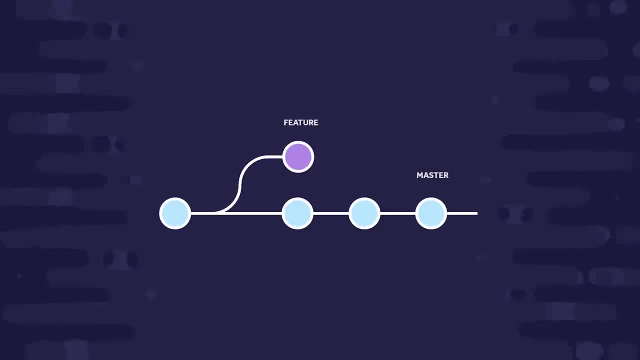 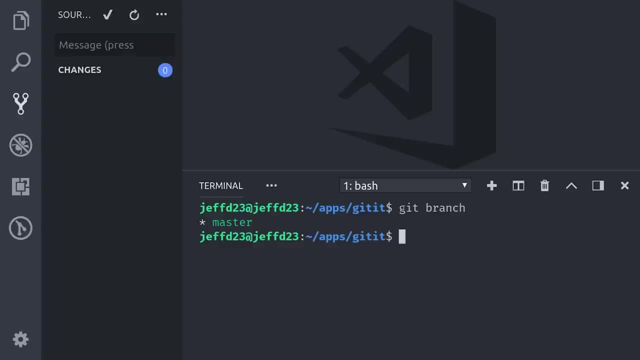 or you want to experiment with a new feature. What you'll typically do in git is create a new branch based on your most recent commit and go and fix the bug on the separate branch and then merge it back into the master branch once it's ready. 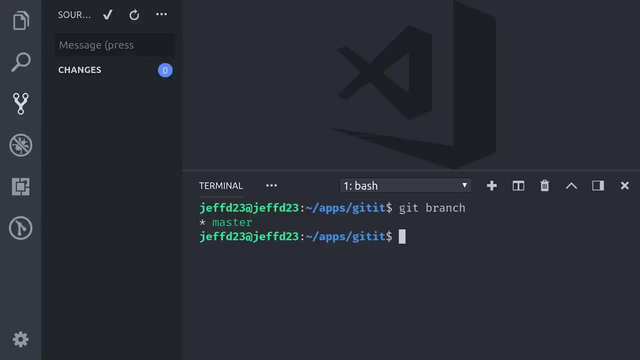 This means we can have multiple developers working on the same codebase on their own branches without stepping on each other's toes. You can see all the current branches in your codebase by running git branch, Which for us would just be the master. You can switch between branches in git by running the checkout command. 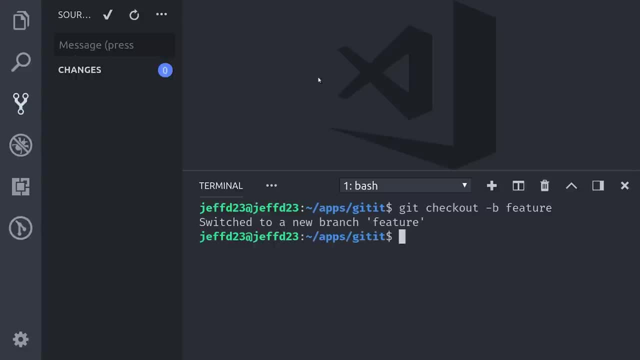 In our case the branch hasn't been created yet, so we'll go ahead and create it by using the b flag and we'll give it a name of feature. So now any code that we write in here will be isolated to this branch. Now we can fast forward into the future, and you'll see, I've written a bunch of code in. 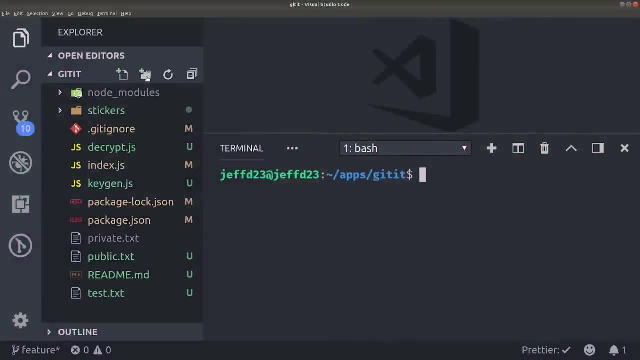 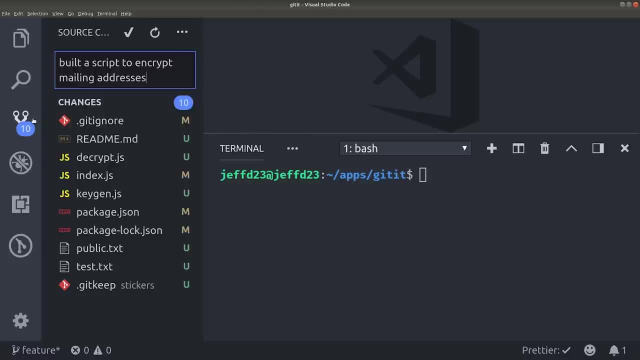 this branch. So currently this code is just sitting in the working directory, so I need to commit it to this feature branch. This time I'll run my commit directly in vs code And then we can switch back to the master And you'll see that all of our new files disappear and we're back to the original. 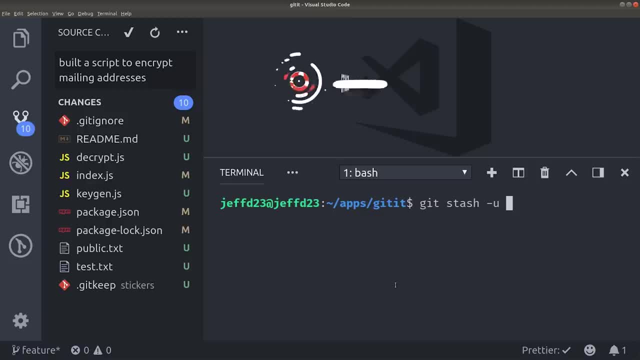 state on the master. At this point, I'd like to point out that you don't necessarily have to commit your files before switching to the master branch. There's another mechanism to save your work in progress. If you're working on something that's half finished or experimental, you can use a command. 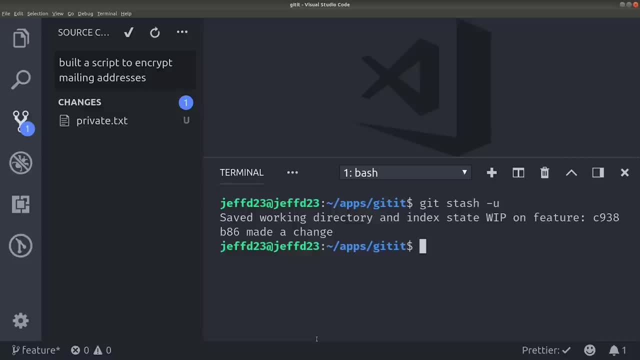 called git stash. This will save all of your current changes without committing them, and then revert back to a clean working directory. Then later at some point in the future, when you want to get back to work, you can either pop or apply the changes anyway. 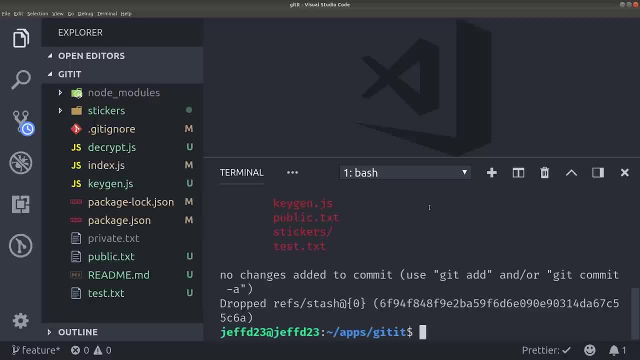 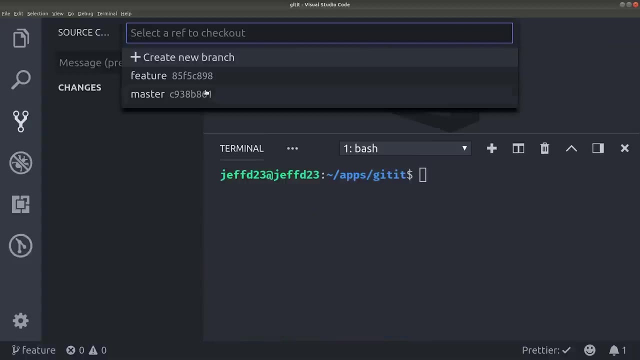 So, just like it sounds, you're stashing away your current changes to be used at some later point. So stashing is just a handy thing to know and an alternative to committing your code if you're not quite ready to do so. In our case, we're all done building our feature, so what we want to do now is merge that feature. 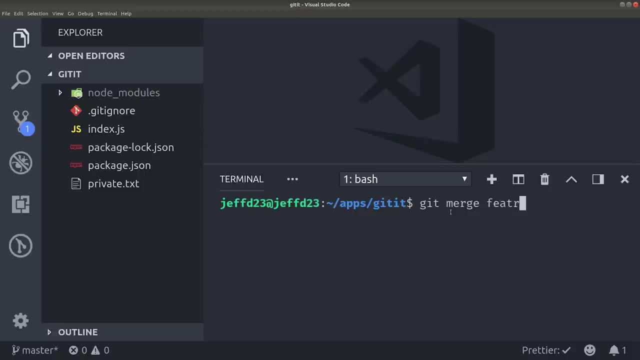 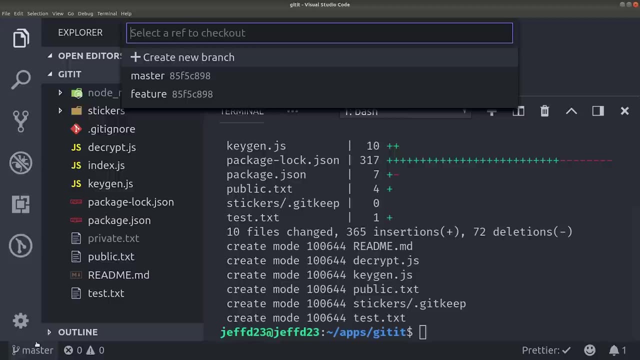 into the master branch. So now we'll go ahead and check out the master branch And then if we run git, merge with the name of our feature branch, it will merge the latest commit from the feature into the master And you'll notice the commit. 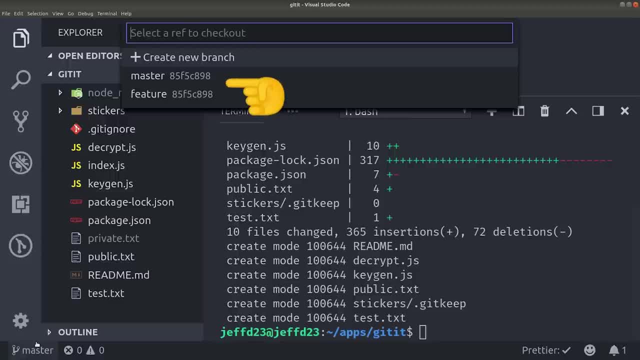 id is the same for both the feature and master branch, So that was a pretty simple use case. but merging is the place you're most likely to run into problems, because you might be working on a feature branch and then the master branch has changes that eventually lead to merge conflicts. 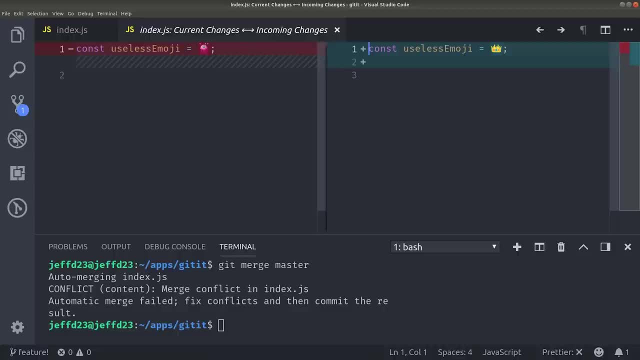 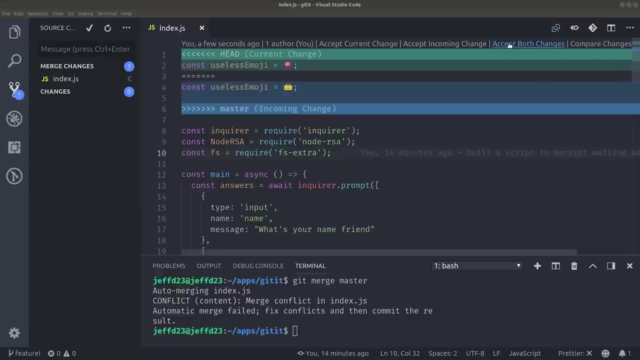 On the left we have a line of code that we implemented in our feature branch and then on the right we have a new change that happened in the master branch while we were working. that affected the same line of code. So merging these files is not possible out of the box because git doesn't know which. 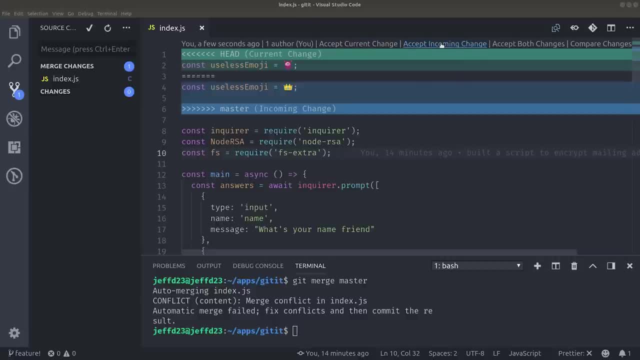 change to use vs code will give you some options to resolve these conflicts. For example, you might accept the current change, accept the incoming change, or both. When you run into a conflict, you'll want to first review it and then a lot of times it's. 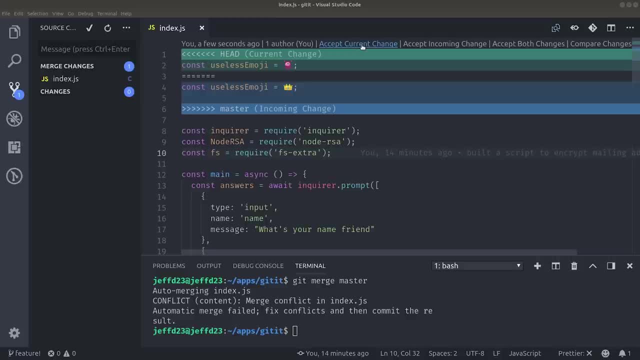 best to just abort the merge altogether and fix the files manually. I already mentioned that it's a good practice to implement a lot of small commits because it's easier to fixate conflict on one file as opposed to 100 files. Then in the previous example we merged a feature branch into the master branch. 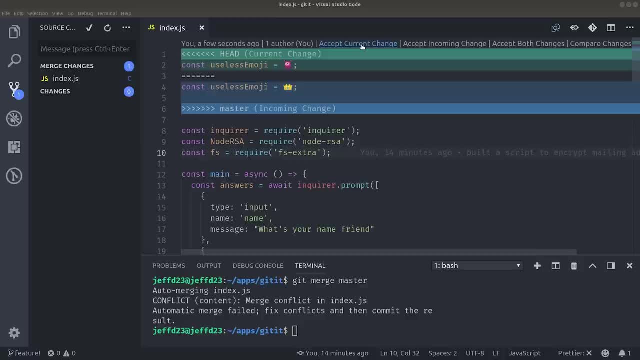 But a lot of times when you're working on a feature you'll want to merge the master branch back into your feature to get the latest code, Because if something on the master branch changes, it means someone could have been writing code in the same place that you're writing code or there might be some breaking changes. 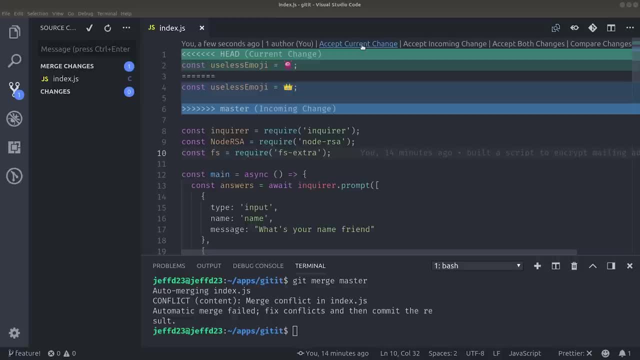 that change the way your feature is going to work. So if you're working on a feature for an extended period of time, you'll want to merge in the master branch anytime it changes, or maybe once a day if it's a really active repo. Now there's one last pro tip that I want to give you. that's related to merging. 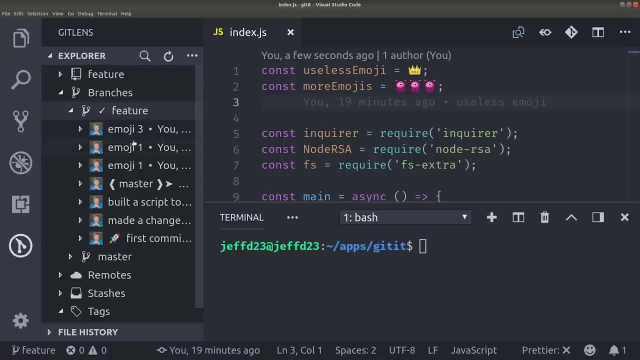 A lot of times on a feature branch you'll create a lot of different commits and these commits are kind of irrelevant to what's going on in the master branch. You can see here that our feature branch is three commits ahead of our master branch and it has a bunch of comments about adding useless emojis to the code. 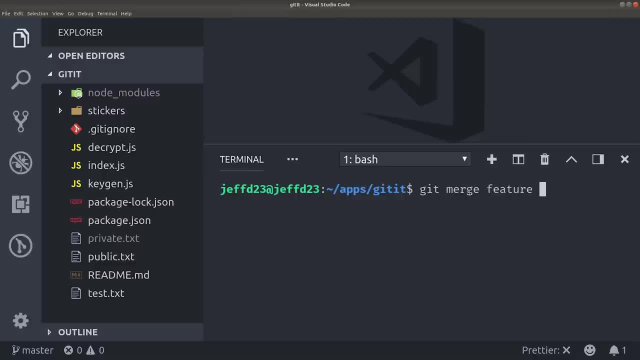 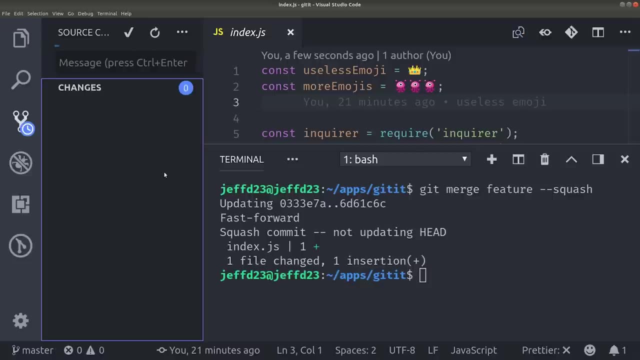 Instead of merging all of these commits into the master branch, you can use the squash flag to squash them down into a single commit when you do your merge. This will keep the change history nice and concise on the master branch but still preserve all of the original commits on the feature branch itself. 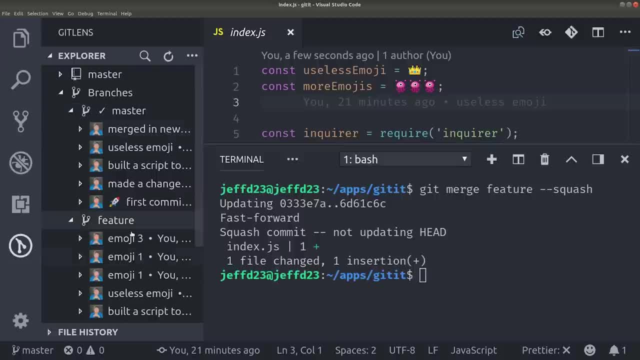 When you merge with the squash flag, it won't actually change the head commit on the master branch, so you'll need to add an additional commit on your own that says something like merged in feature branch and that gives us a nice compact change history on the master. So now that we know how to do all this git stuff locally, let's see how we can do it. 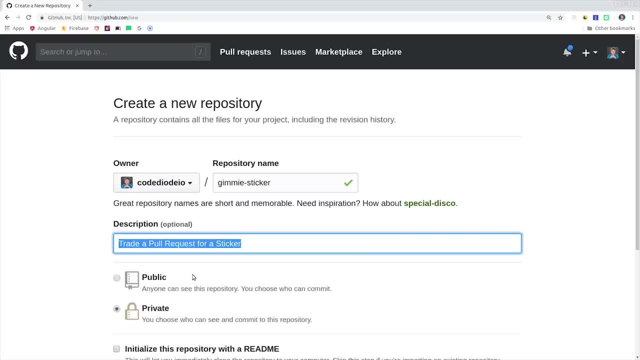 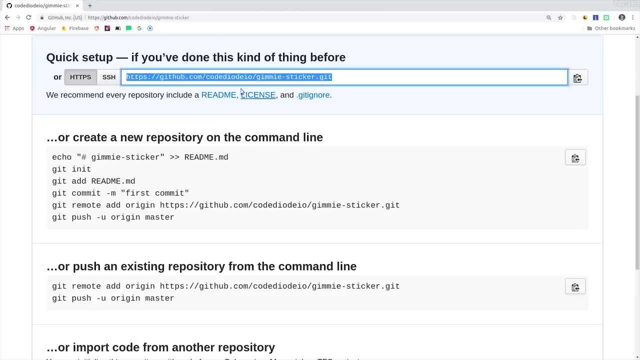 remotely with github. Pushing a repo to github is actually really easy. First we just need to create a repository on github and then it will give us the commands to run to push our code to this location. The first command is git remote, which connects your local code to this remote repository. 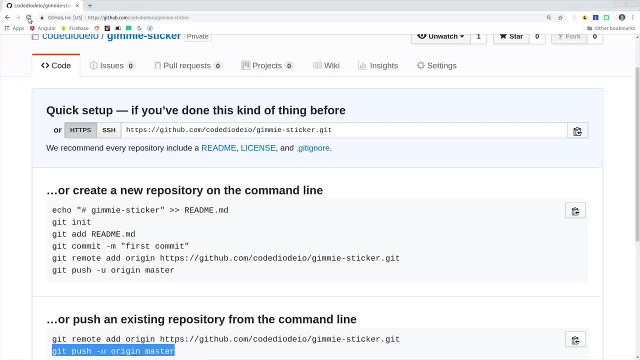 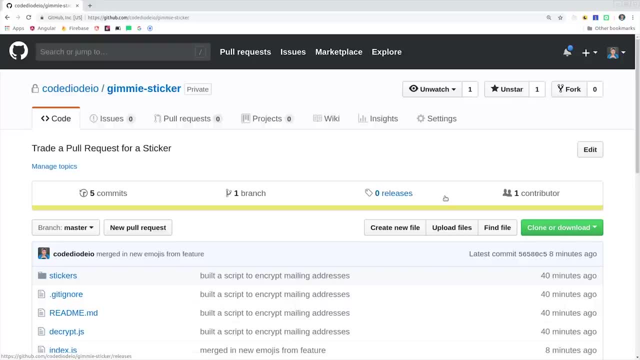 which will actually push the files to the remote repository. So if we run the commands and then refresh the page, we should see our code is now on github. That was super easy. but the next thing I want to show you is how to take someone's existing code, fork it, create some changes and then create. 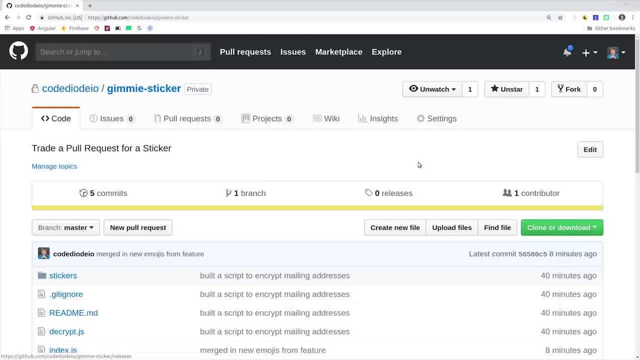 a pull request to merge your code into another person's project, And that's exactly what you'll need to do to get the free sticker. So this is the typical pattern that you'll see when contributing to any open source project. Step one is to fork the existing project. Forking will. 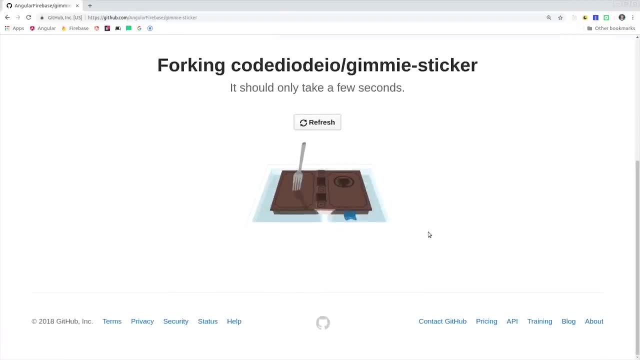 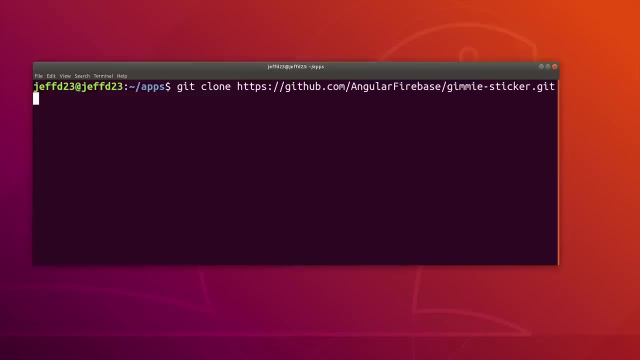 allow you to copy the code from the source and make it a repo under your own github account. After you fork it. you'll then want to clone your fork to your local machine so you can start making changes to it. The git clone command just allows you to copy the code from a remote repository to 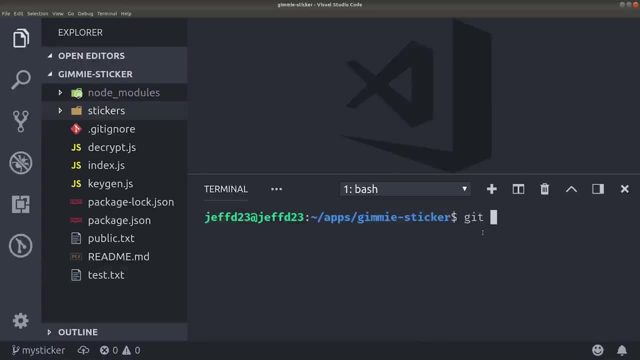 your local computer. Once you have that cloned, you can open it up in vs code and in this case here you'll first want to run npm install to install the dependencies. Then you can run git checkout, flag b with my sticker as the branch name, which again will create and move you into this new 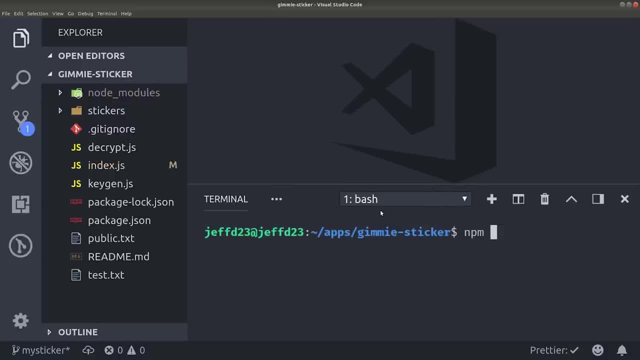 branch And then, after you've done that, you'll want to run the next step, which is to run the npm run address command. I've added a special command to this repo called npm run address, and that's going to prompt you for the information that I need for your mailing address. 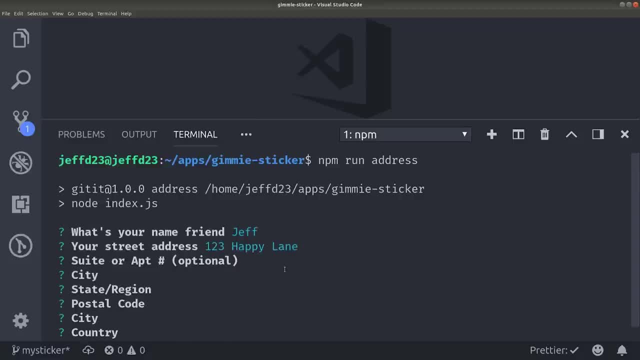 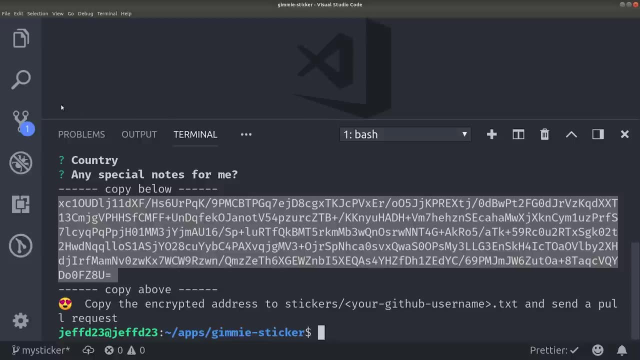 When you're done with that, it will print out an encrypted base64 string. From there you'll go into the stickers directory and create a new file that's your github username dot txt. Then you'll copy and paste this encoded string into that file. So just a side note on security. your address is: 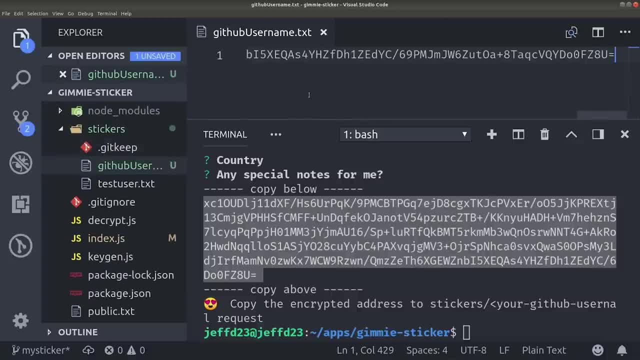 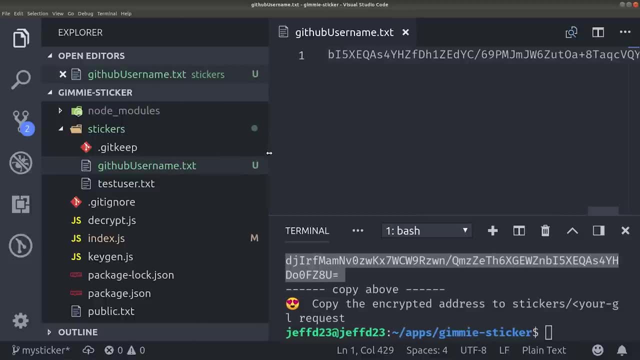 going into a public repo, but it's encrypted with the rsa algorithm. This means that you're able to encrypt data with the public key, but I'm the only one with a private key that can decrypt it. I have the private key on a thumb drive, which I'll destroy after this giveaway and hacking the private. 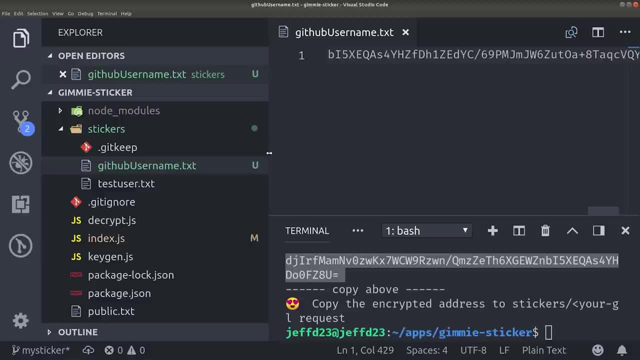 key by brute force is essentially impossible. So unless someone physically steals the private key, your address should be safe in this public format. but I do feel obligated to give you that disclaimer first. Now go ahead and save the text file, then run git add and git commit with whatever message. 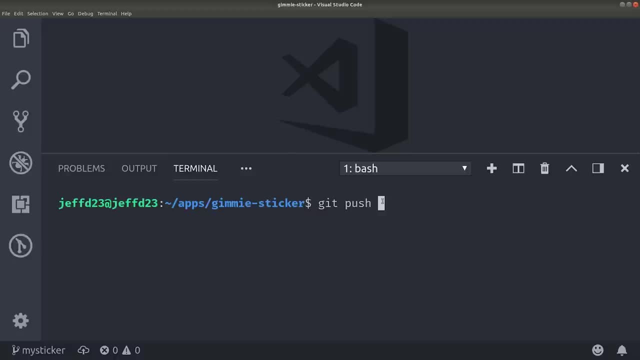 you want to put in there. Now we have all of the necessary changes committed on our local machine. First we need to create a new pull request. For that we can just say git push origin with the branch name, and that will push the branch to github. Then on github you'll see the option to. 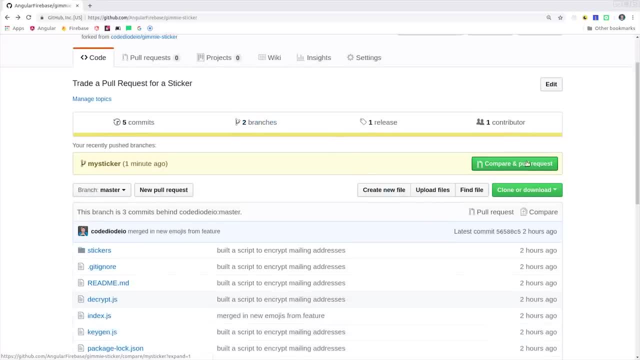 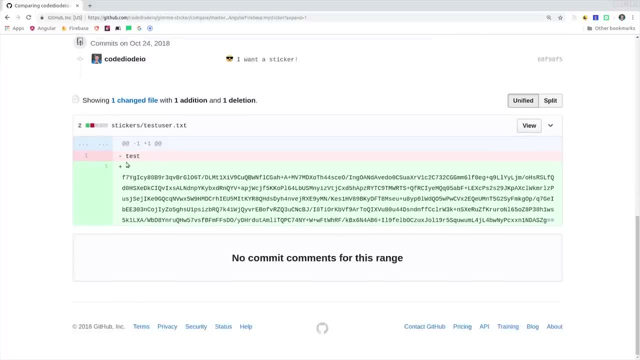 create a new pull request. A pull request is just like a merge, but it has the additional step of needing to pull in the remote changes. In other words, a pull request is like saying: pull in my remote changes and then merge them into the master branch. So that's how you contribute to an open. 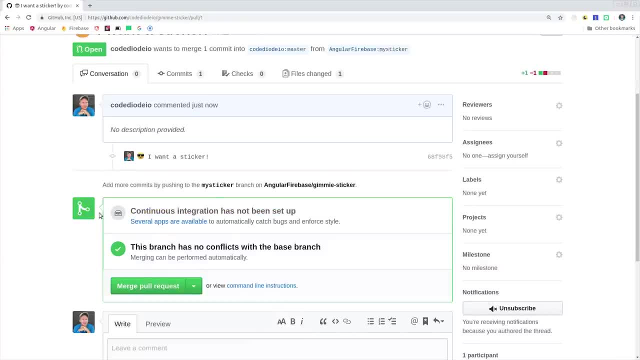 source project. I'm going to go ahead and wrap things up there. Hopefully that leaves you with some of the basic tools needed to contribute to open source software. So let's get started. There's a whole lot more that can be covered on this topic, so let me know what you want to. 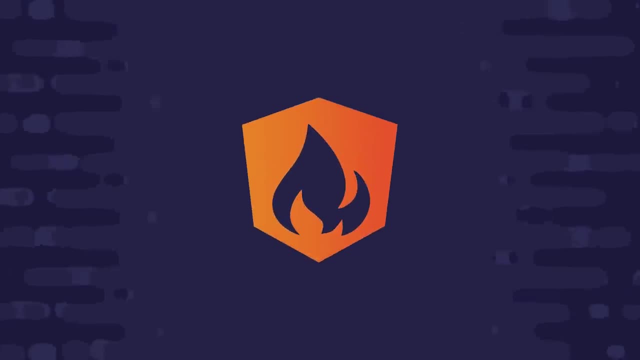 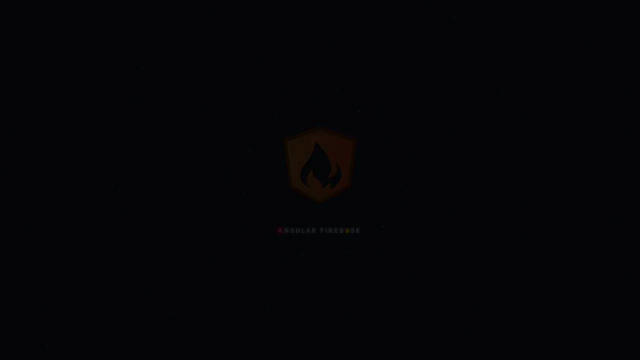 see next in the comments, And if you want to get really good at this kind of stuff, consider becoming a pro member at angularfirebasecom. Thanks for watching and I'll talk to you soon.